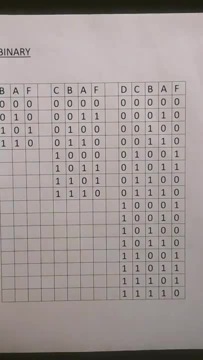 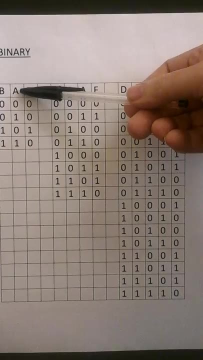 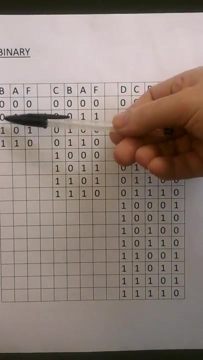 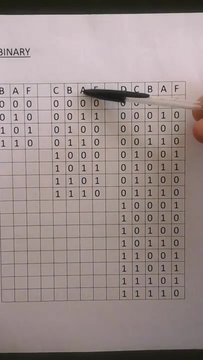 for the two variable function, then the three variable, then the four variable. so we start off with zero one and repeat the pattern down. that's input variable A, input variable B. we repeat the pattern but in groups of two. so two zeros followed by two ones for a three variable function variable. 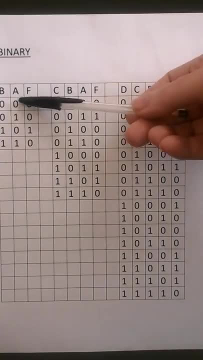 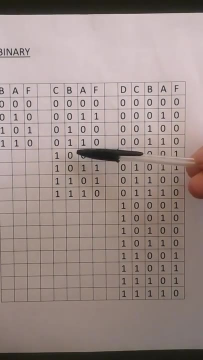 A follows the pattern: zero, one, zero, one again. it's similar pattern to this all over and all the way down. variable B follows the pattern: zero, zero is pulled by two ones all the way down and repeats the pattern. the variable C: you have four zeros, four by four ones, there's a four. 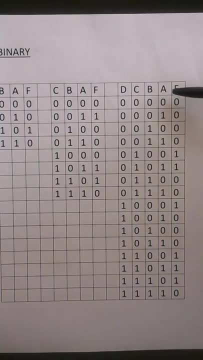 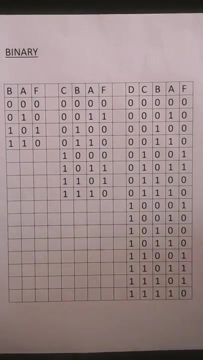 variable function here: F, A, B, C, D. A follows a pattern- zero one and repeats. b follows the pattern- two zeros by two ones and then repeats c, for follows the pattern by four ones, repeats. and D follows the pattern: eight zeros, power, followed by eight ones. now, instead of writing all combinations this way, this method allows you to generate. 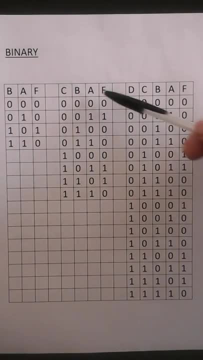 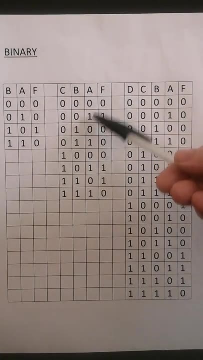 all input combinations, and starting with one, the column to the left is twice the number of consecutive zeros and ones as a column to the right. so here you have one zero, then two zeros and four zeros, and then the pattern repeats. here you have one zero followed by two zeros. 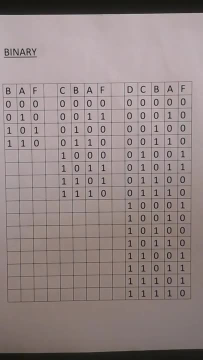 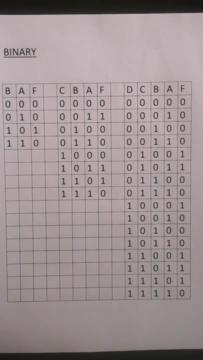 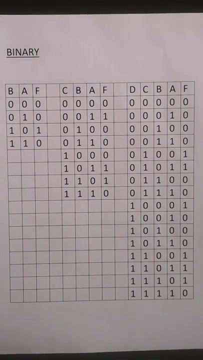 powered by four zeros followed by eight zeros. if you had a variable a here for a five variable function, you would have sixteen zeros followed by sixteen ones of. okay, that's two variables. let's just mention f in each case was arbitrarily chosen just to represent what a function may look like. it consists of zeros and ones for binary base two. 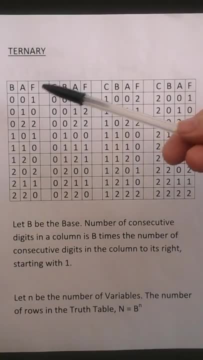 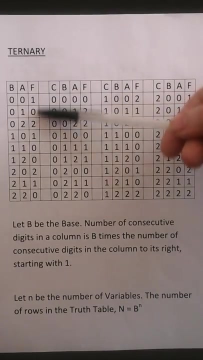 here you have a ternary functions base three. here we have a two variable function and a three variable function here i've split this into three because i couldn't fit all the listings in one true table, so it was split into three just over a four paper. here we have f for two variable function. 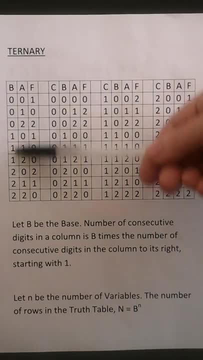 consists of zero ones and twos and input combinations a and b. now a follows the pattern: zero one, two, zero one, two, zero one, two and b follows the pattern: three zeros full of zeros, two zeros full of zeros and b. now a follows a pattern: zero one, two, zero one, two, zero one, two and b follows the pattern: three zeros full of zeros and b. 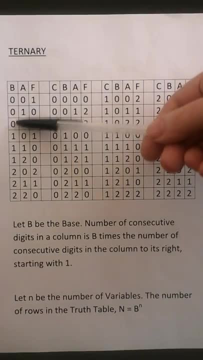 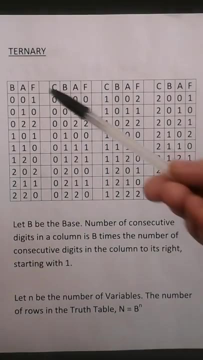 a follows a pattern 0, 1, 2, 0, 1, 2 &. B follows the pattern between 0% & f, 4x, f4x, zeros, followed by three ones, followed by three, twos again. the rule is you start with one of each one and then you repeat it three times. so one zero there three. 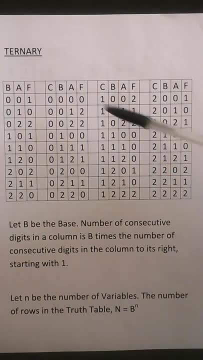 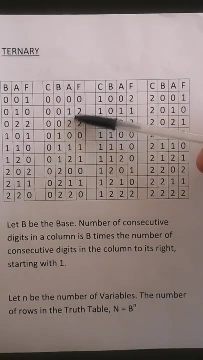 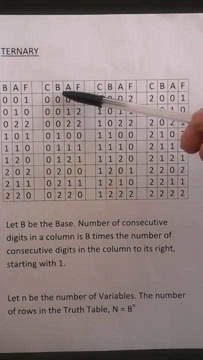 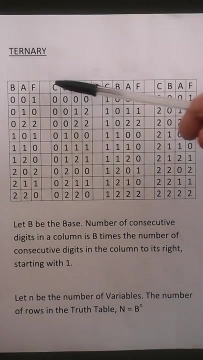 zeros there, followed by three ones, followed by three twos. for the three variable function ABC, the same pattern arrives: zero one, two, zero one, two, zero, one, two. same deal here. Pattern B: there's three zeros, three ones and three twos. the same for pattern B. here and for column C, it's nine zeros, followed by: 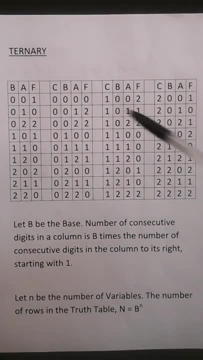 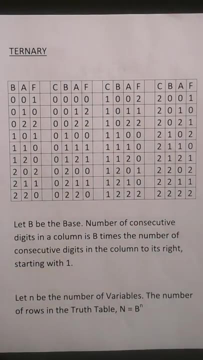 nine ones followed by nine twos, so again you start with one. then it's three times the number of consecutive digits. so 3 there, 9 there. Ok, so if you let B be the base, the number of consecutive Penn System column is B times the number of consecutive different digits in the 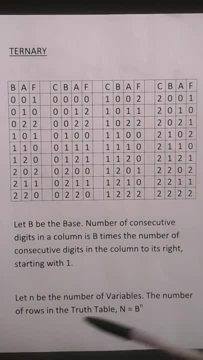 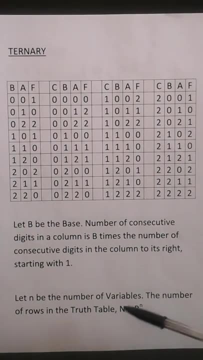 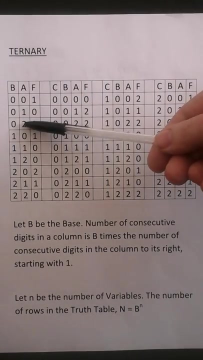 column to its right started with one, which is what I've said here. so let n be the number of variables: ABC. three variables, AB: two variables. the number of rows in the truth table is n. n equals B to the n. so basically, three squared two variables. n equals two, nine rows of the truth table. here we have three base. 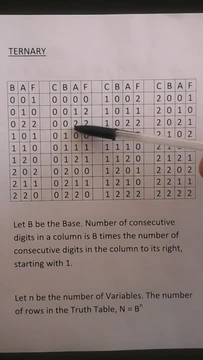 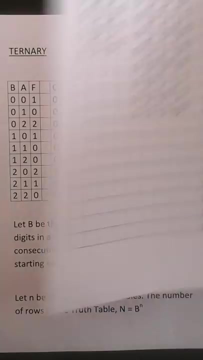 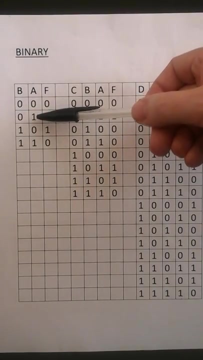 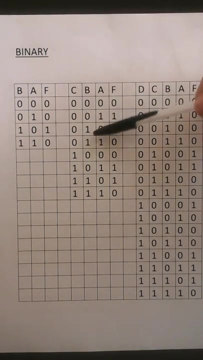 three, three variables, three, three digits: 0, 1, 2, n equals 3, 3 inputs. so 3 to the cubed is 27 rows of the truth table. yeah, and if we go back to the binary one, we have binary 0, 1, 2. base is 2, 2 inputs, 2 squared is 4, 2 cubed is 8 for 3 inputs. 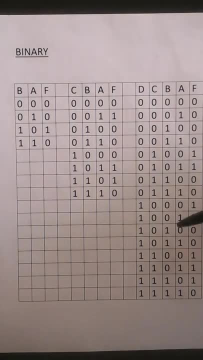 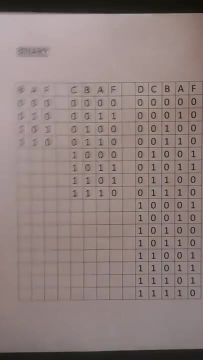 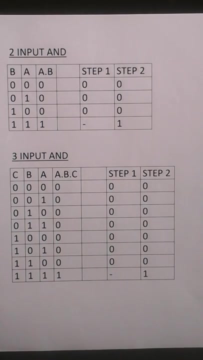 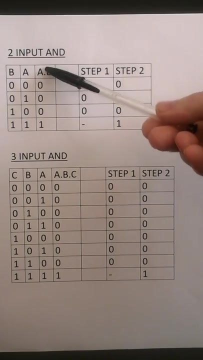 and 2 to the power. 4 is 16 for 4 inputs. the 5 variable input would have 32 rows, the combination of the truth table. okay, now we get on to the Boolean functions themselves. here we have an and function input, say B, generated as showed before for a binary truth table, and the amp of instead of F. 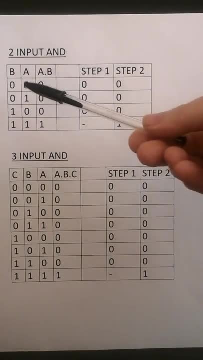 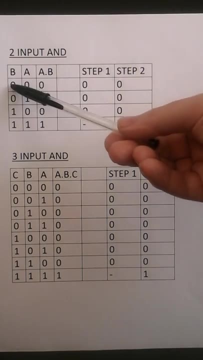 we have a and B, which is the, and function the variables A and B. and the way you complete the truth table is to first look at the inputs and any time you get a 0 on the input, on any of the inputs, you get a zero. 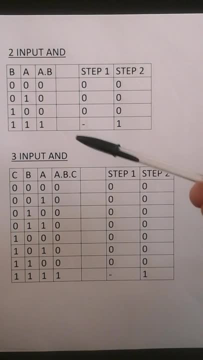 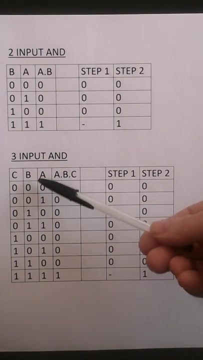 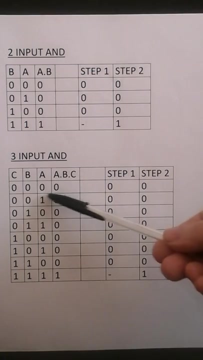 zero on the output. that's step one. and step two fill in the remaining space with a one, so one and one equals one for a three input function of ABC input variables function is a and B and C. step one: look for these zeros on any of the. 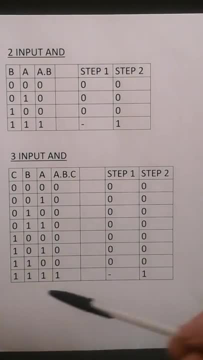 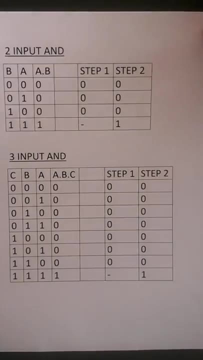 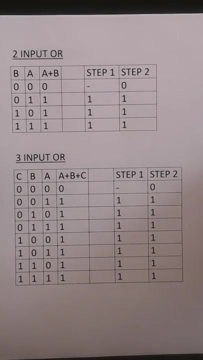 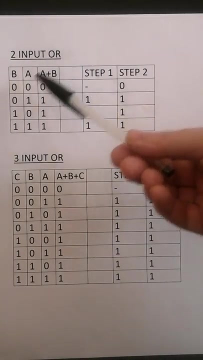 inputs and put it on the output. and lastly, the only combination left is when all the inputs are one, which the output is a one. here we have an R function for two variables to input: R, a and B. here we have the input combinations a and B as. 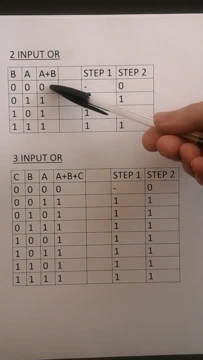 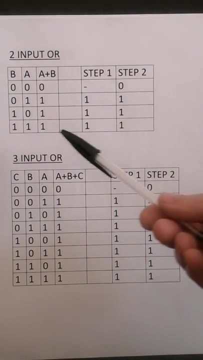 shown before here, the function is a or B, which has this output combination. so the way you fill in the truth table is to look for the ones on any of the inputs and fill the output with a one at step 1 and step 2. you fill the remaining output with a. 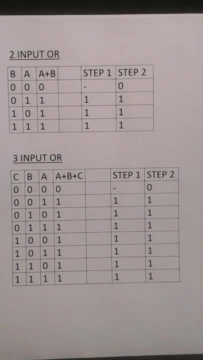 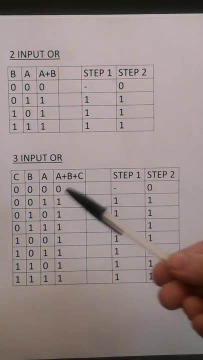 zero. that's when all inputs are at zero. for a three input: R inputs a, B and C and C variables got A or B or C. you look for a 1 on any of the inputs and you fill that with a 1. that's step 1 and then step 2. you fill in the remaining 0. 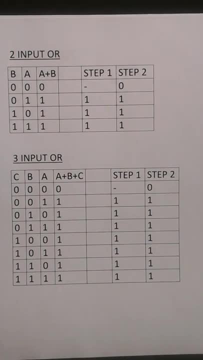 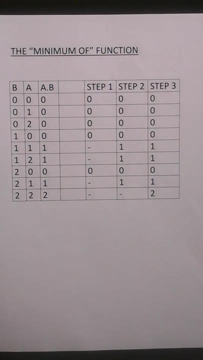 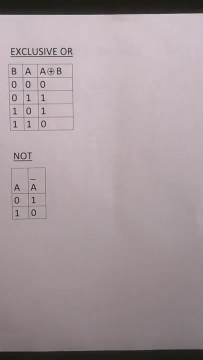 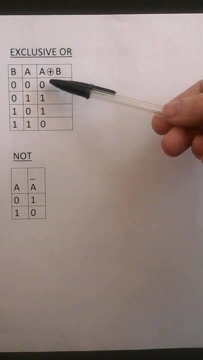 when all the inputs are 0. Here we have an exclusive off function. now these functions are generally made in electronics terms with two inputs only. so I have the input variables A and B here and the output is a, one if, and only if, one output or the other output. 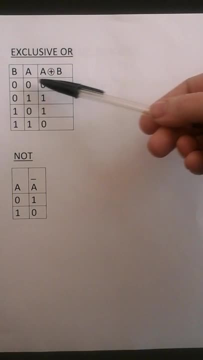 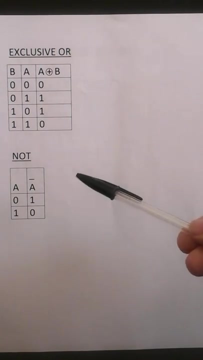 is a one, but not both at the same time. so zero, they're one, they're one there and zero, and here we have the not function, which is unary operator. one input in reply. in reply to 0, 1, you get the output 1, 0. so 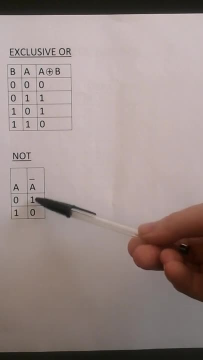 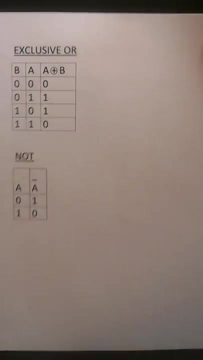 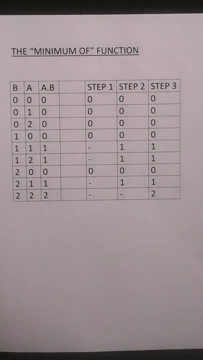 basically, it's not whatever that is isn't the other, it's not a. not a is signified by a bar of the top. now we go on to ternary functions, which is base 3, base 3 logic system by those system. those functions have described earlier. 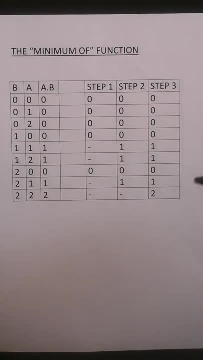 for binary with Boolean, the and the arts, because we've are, they're not, they'll. boolean functions. these are ternary functions, these and multiple valued logic functions. multiple valued logic describes any logic system with a base of 3 or more, and binary is base 2, so we have the. 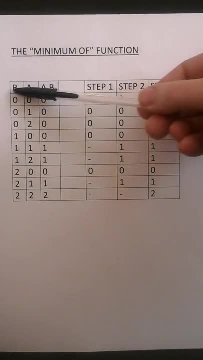 minimum of all the functions and the binary is base 2, so we have the minimum of function here. you have generated a and B, the truth tables 0, 1, 2, 0, 1, 2, 0, 1, 2, 3, 0, 3, 1, 3 twos and we have the output here for a and B got a minimum function. 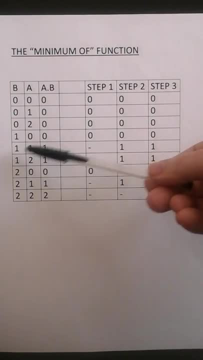 minimum function because the output takes a minimum whatever is on its inputs. so it's a similar process to generate the, the output of the function. step on: look for zeros on the inputs and fill them on the output and leave the rest blank. step 2: next, look for the ones there, fill them in. lastly, look for 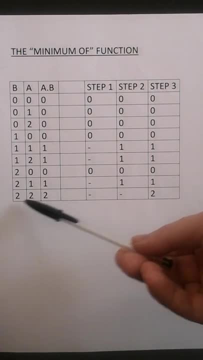 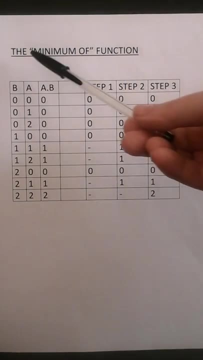 the twos for the minimum function. the two will only care when all the inputs are on to, so I called it a and B, but really it's a minimum of function. it's the ternary minimum of function, the and function in boolean in binary would be the binary equivalent of the. 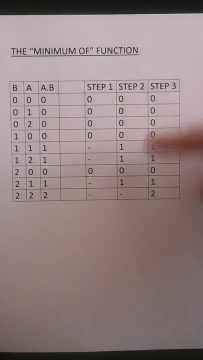 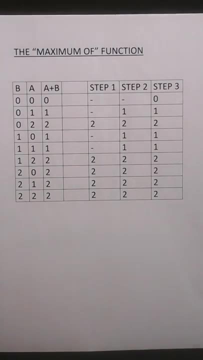 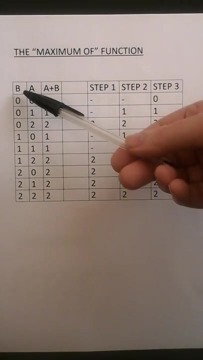 minimum of function. so it's a similar process to generate the output of the truth table. you have the maximum function. this is equivalent to the well, in the binary case the maximum function is the all function. so we have inputs a and B, maximum of B, ALB if you like- and we have the input, say 0, 1, 2, 0, 1 0, 1 2 and the 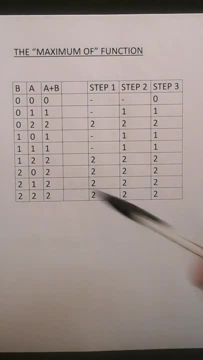 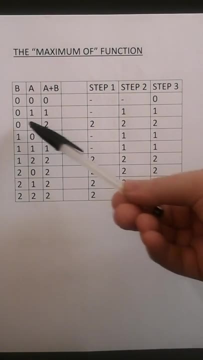 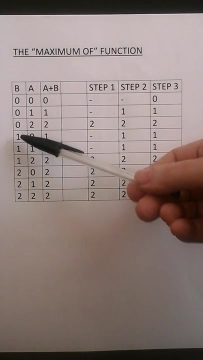 outputs there for B: 0, 0, 0, 1, 1, 2, 2, 2. now to fill in the maximum function. you look for twos on the inputs and you fill in the output with a 2 whenever there's a 2 on the input. that's step 1, step 2. next you look for the ones here for the 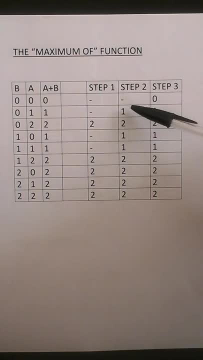 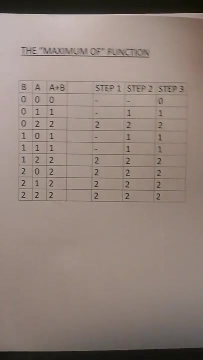 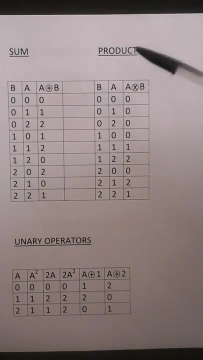 remaining outputs that aren't a 1 and being filled in. sorry, there a 1 and next you fill in the last input, which is a 0. 0 happens when all the inputs are 0. here we have the summing product function. this is this is read Muller logic for. 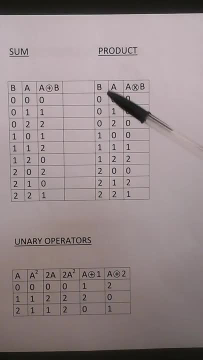 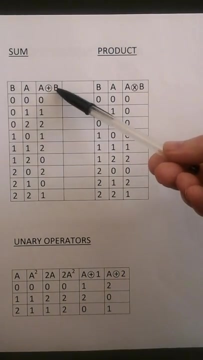 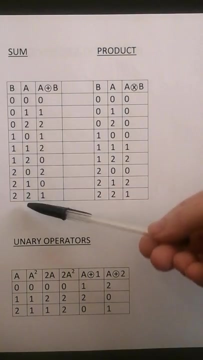 base three ternary read Miller logic relies on the sum product functions to generate the output of the truth table to generate a function. sorry. so here we have a two variable input sum function: a and B, a plus B. sorry, there is the, the input variables a and B. that's the truth table for it and, as you can tell, it's. 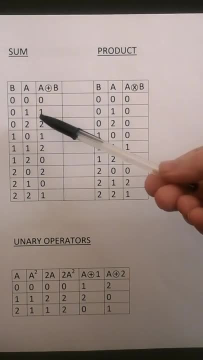 just a straightforward sum modulo 3. so: 0, 0, 0, 0. 1 is 1, 0 plus 2 is 2. 1. 1 plus 1 is 2, 1 plus 2 is 3, which is 0 modulo 3. so using the sum modulo 3, rate arithmetic: 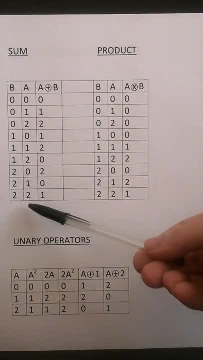 to their 0 again, and 2 plus 2 is 4, which is 1 modulo 3. here we have the product function generating the same method of the input variables and the times, as you would expect, to 0 anything. 0 is 0 anything times 0, sorry, 0 1 times. 1 is 1, 1 times. 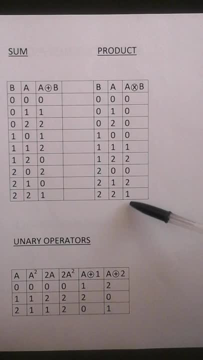 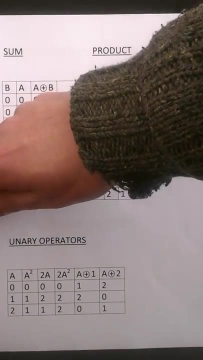 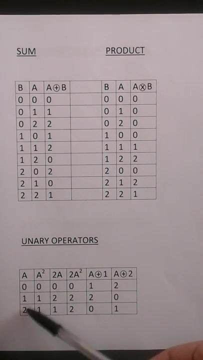 0 is 2, and here we have 2 times 2 is 4, which is 1 modulo 3. here we have some unary operators, we have a squared which is a times a, so 1 times 1 is a 1, 0 times 0 is a 0, 2 times 2. 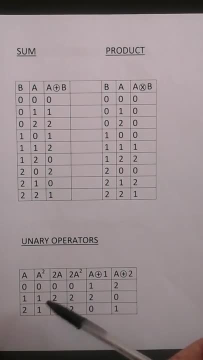 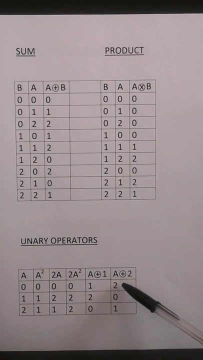 is a 1. here we have twice a, which is 0 to 1, twice a squared 0 to 2 a plus 1, 1 to a which is 1 plus. this is the successor function and this is a predecessor function in response to 0, 1, 2, yet 2, 0, 1, 4 a plus 2. 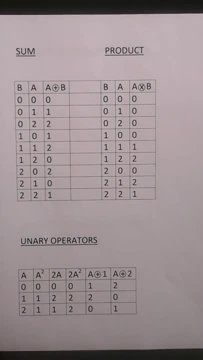 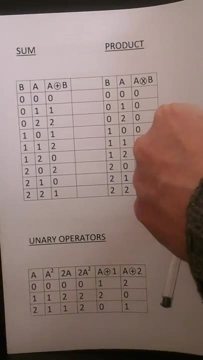 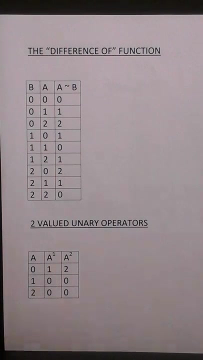 so that is for read more logic. base three: ternary: here we have the difference of function. I've put this function in only because it's useful for one purpose: the output gives the difference of whatever is on its inputs. it's only a two input function, so why do it? well, for a start it's useful. 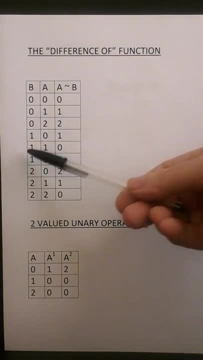 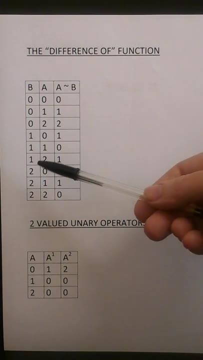 when the for comparing when the inputs are equal, because in each case the difference will be zero. so, as you can tell, the output is just the, the difference between the two inputs, ignoring the the sign. so a minus B, sorry, a minus B, for example, would be one minus two minus one, but ignore the sign, so it's one. so 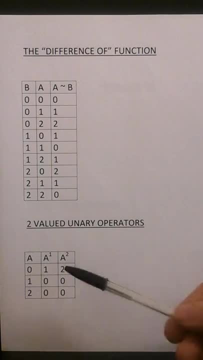 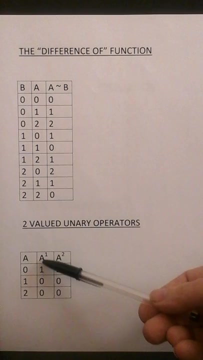 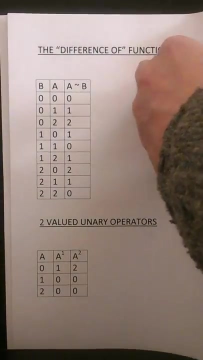 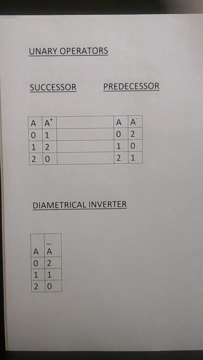 two valid unit operators. this is for a ternary algebra based on these operators, which are two valued. basically the output: a one is a one when a zero is zero and zero otherwise, and a two is a zero is a two, one is zero and zero otherwise. so here we have the unit operators which are with them, ternary, multiple-valued algebra. 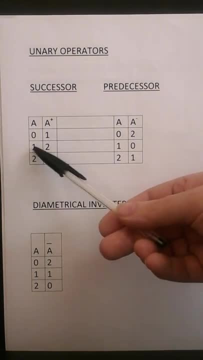 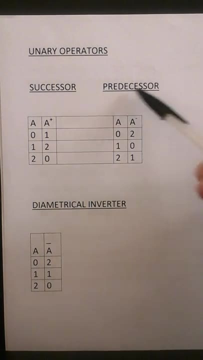 successor a just adds one to the input and add one in, adding one to two modulo three: zero. here's a predecessor function which takes one away from the input. here and adding taking one away from zero equals two. one away from one is zero. two away from one.